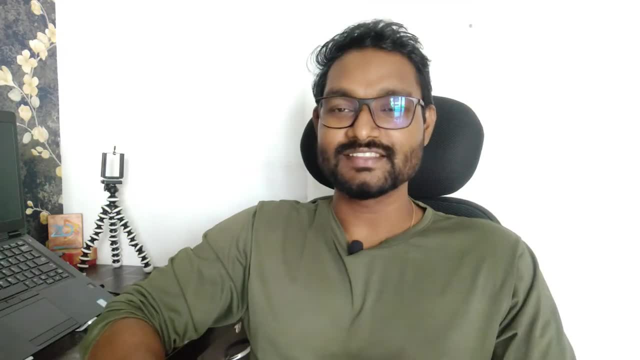 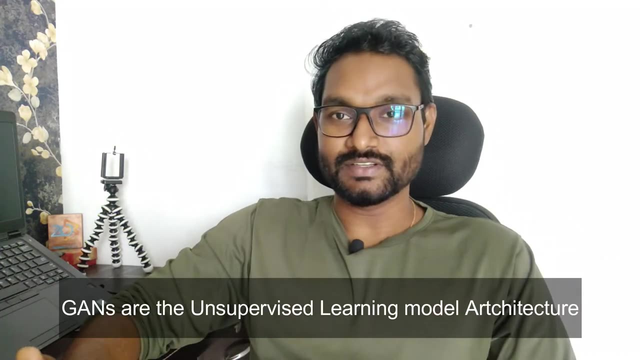 machine learning. Okay, so now let's talk about GANs. GANs are the unsupervised learning model architecture. You must be aware about the supervised learning, where we pass the data along with the labels. our model learns from that data. 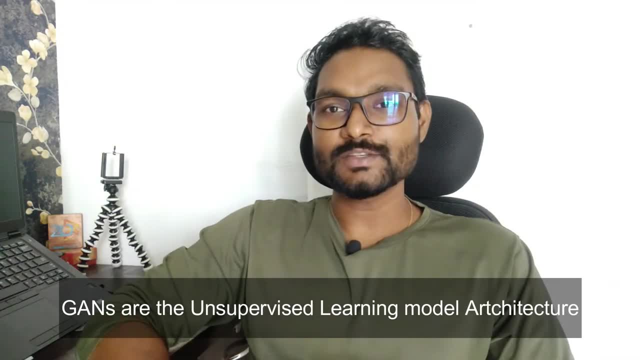 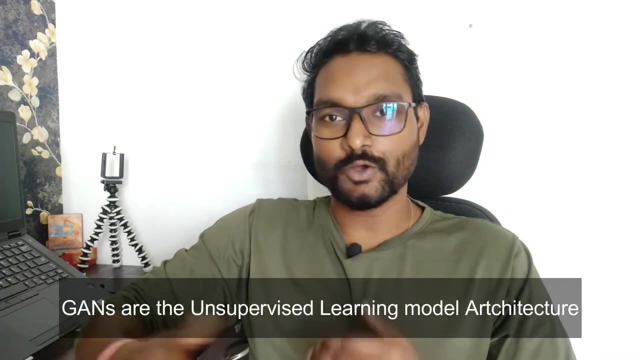 and labels and then do the classification. In unsupervised learning we just provide the data and machine learning model learns the different features by themselves and after that, based on the similarity or relationship between the features, it groups down this data and into the different clusters or the groups. So this GANs falls under the unsupervised learning. 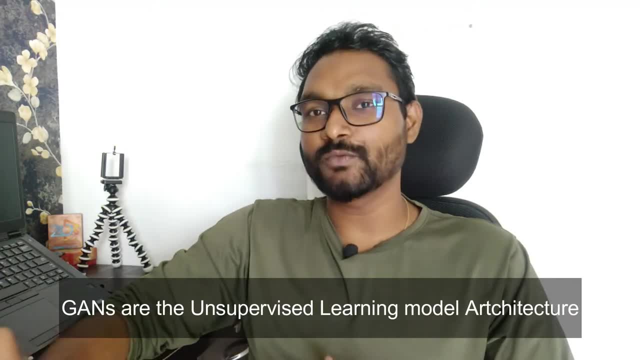 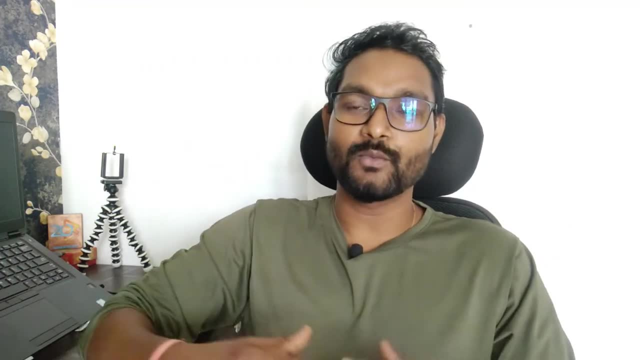 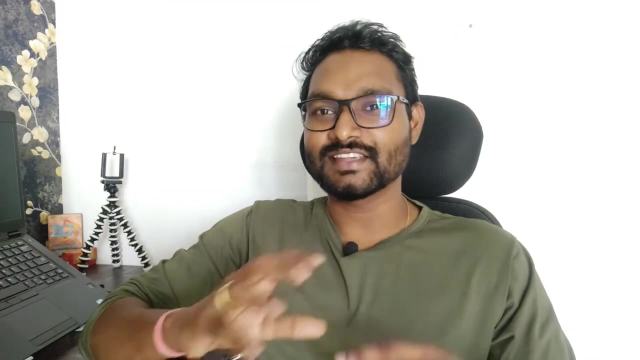 model where we just pass the data and it generates some output for us. So let's try to understand the different applications or what capability these GANs are having and what are all things we can do with GANs, and after that we'll try to discuss in a layman's word what is GANs and inside working. 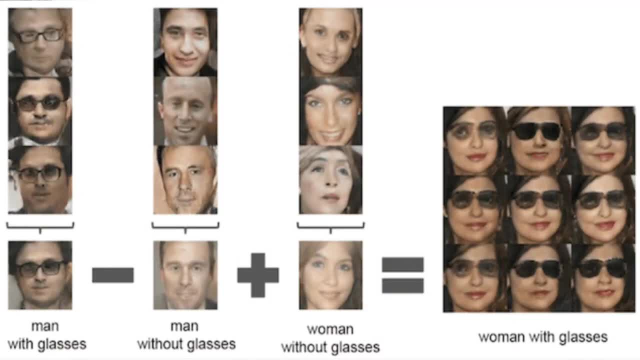 and everything. Okay, here you can see that I have populated one image. on left hand side column you can see that man with glasses, and after that you can see the couple of images of man without glasses. and on the third column you can see that woman without glasses. Okay, so these are different. 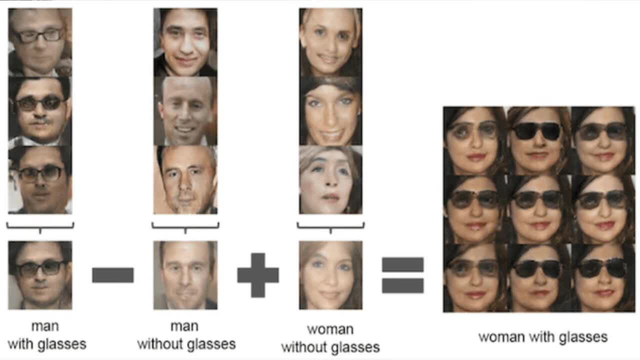 faces of men with glass, men without glass and, after that, woman faces and with the help of that, by using a GANs, we have generated the woman's images with the glasses. Okay, we have combined this main face- main glasses- with a woman face and we have generated the new face image of a woman. 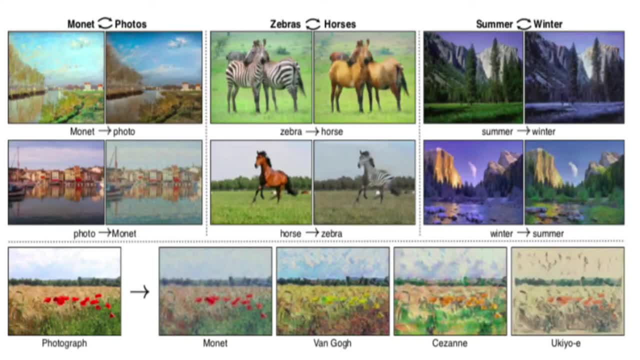 with glasses, Okay. so here we have another image where you can see the different application like. we can generate photos from a monitor, Okay, or we can generate a horse's photo from the zebra's photos, or we can even generate artificial winter photo from the summer photo. One more: 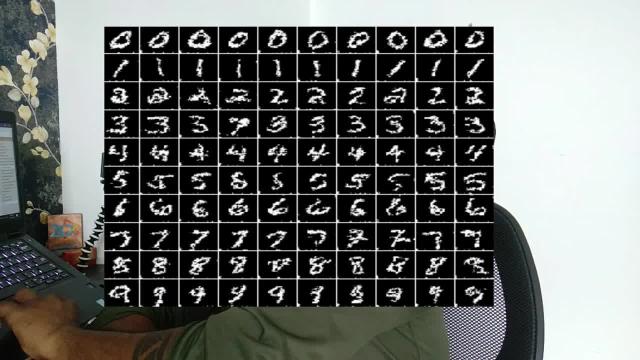 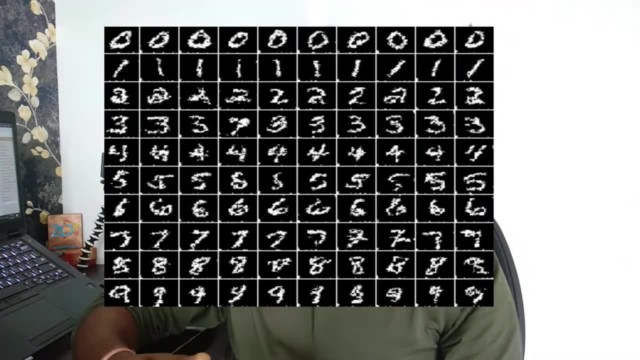 example I'm showing over here. you can see that this is the images of hand drawn characters. Okay, but these are all actually drawn by the GANs. means we have just trained our GANs with the help of MNIST data set, That is, the most common data sets in the computer vision field. That is. 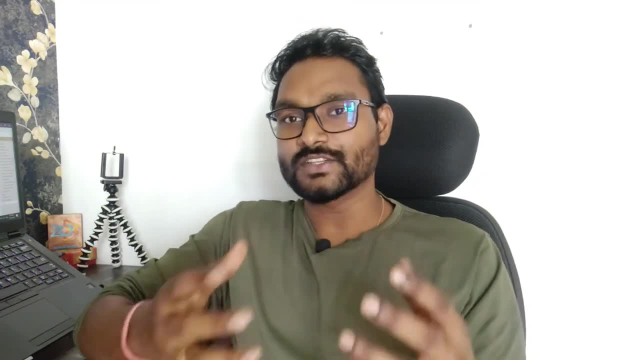 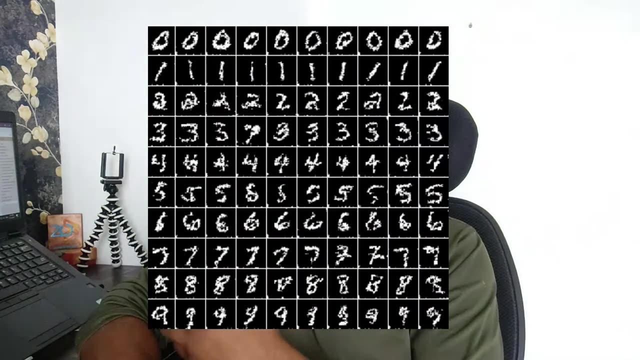 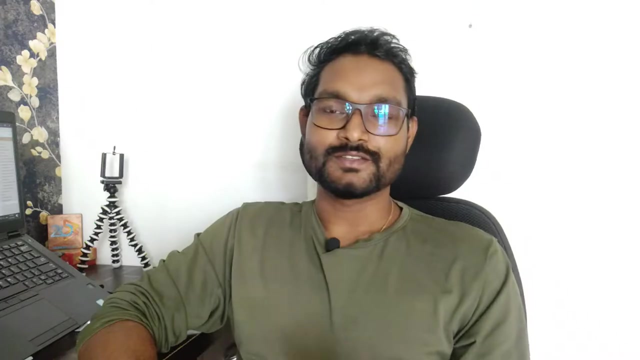 the hand written characters and those we have passed to our GANs, and GANs learn from that images and after that it is generating the handwritten images like that, So you can see whatever the images you have seen on the screen. So these are all generated by the GAN model. Okay, 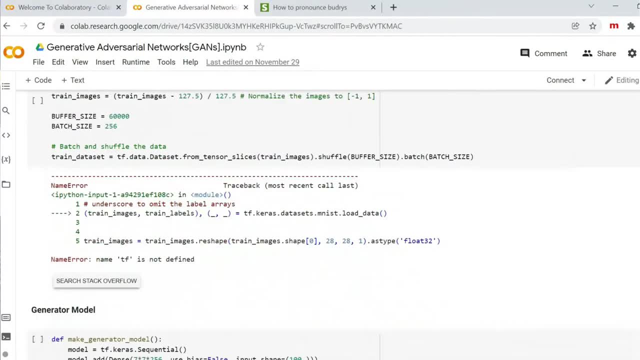 so in our next episode I'm also going to show you demonstration like how we can make use of GANs to apply on the MNIST data set and how you can use them to generate the GAN images. So I and I will see you in second part. Bye, bye. 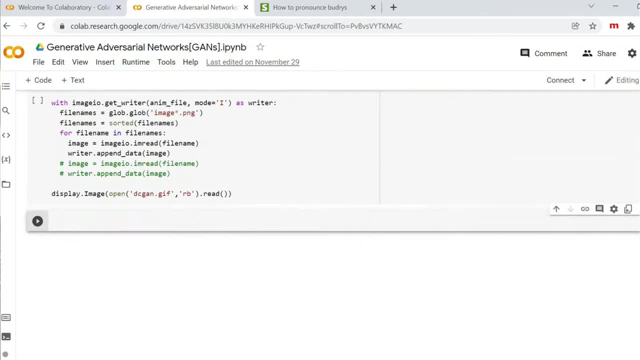 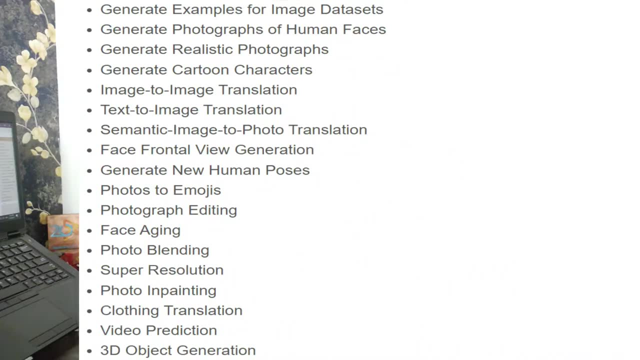 this data set and how you can make use of the GANs to apply on the MNIST data set, and how you can can generate a new handwritten, like an artificial images, with the help of a gans. okay, so coming back, there are different fields in which we can apply the gans. for example, we can generate photographs. 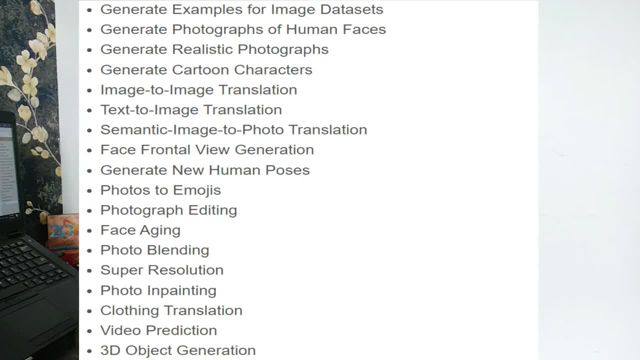 of human faces. we can generate a realistic photographs. we can generate cartoon characters. we can generate one image from the another image, or even we can generate an image from the text that we call it as text to image translation. we can do semantic image to photo translation, face frontal view generation or generating a new human poses. we can do the photos to emojis. we can. 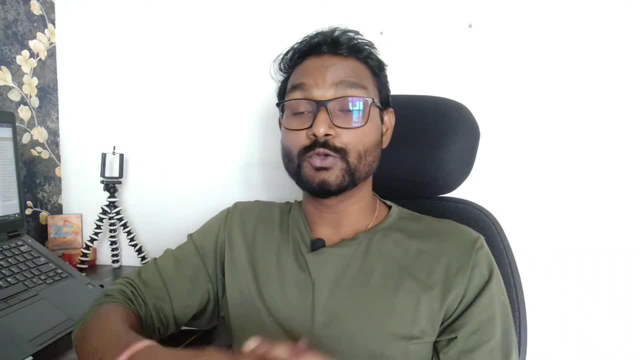 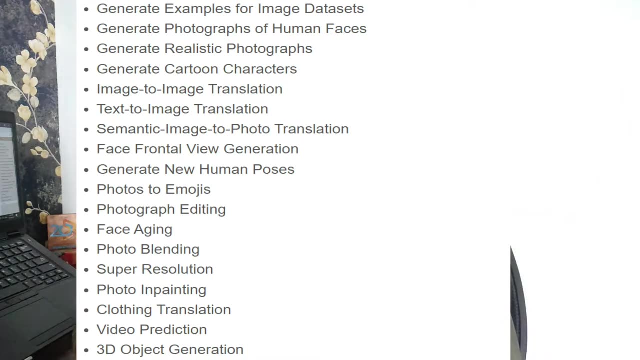 do a photograph editing. we can do the face aging, we can do the blending of multiple photos and generate a new photo. we can do the super resolution, we can do the photo in painting, we can do the clothing translation, video prediction, we can do the 3d object generation. so there are a lot. 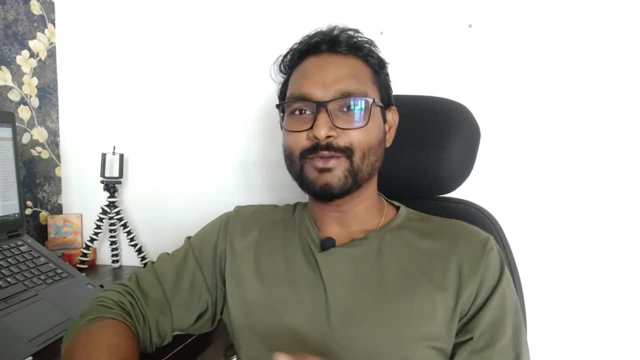 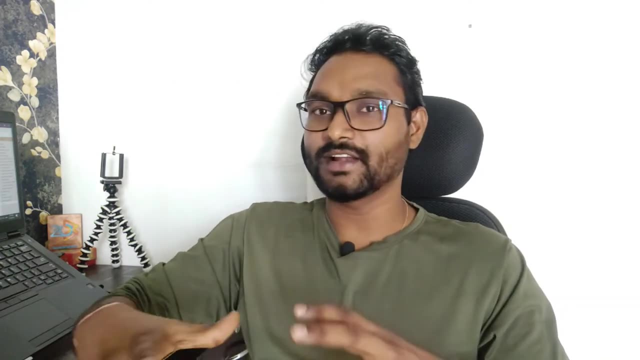 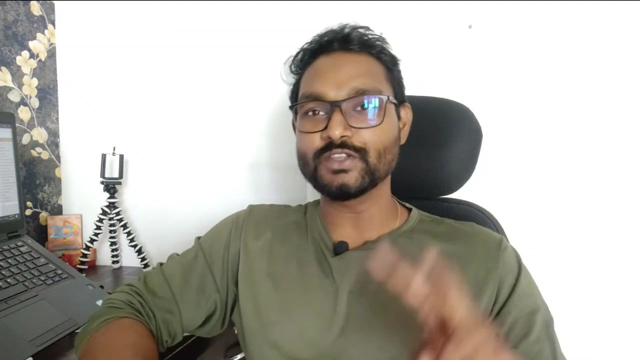 of areas in which we can apply this gans. now let's go and try to understand that. what exactly inside GANs? we understood that GAN is an unsupervised learning model- architecture. but how exactly it works? okay, so before that, let's understand that inside of GAN, we have the two different models. 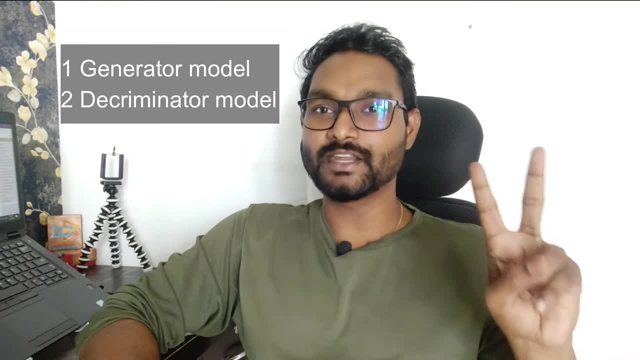 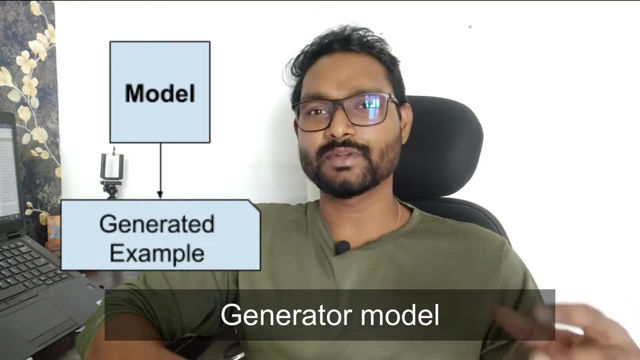 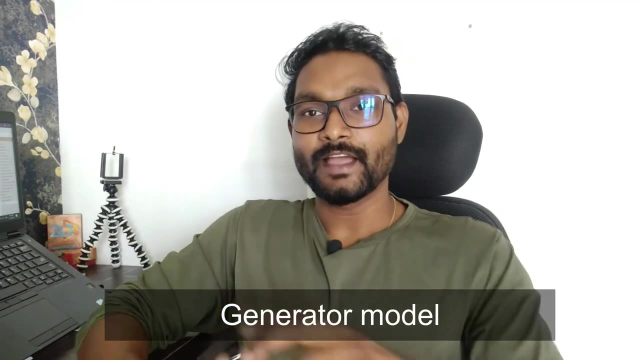 first one is a generative model and second one is the discriminator model. okay, so generator model just generates new image from the random input. okay, so you can take some random input, pass it to generator model and it will generate one artificial, newly generated outcome, and another one is a discriminator model. so discriminator model is responsible for discriminating the output. 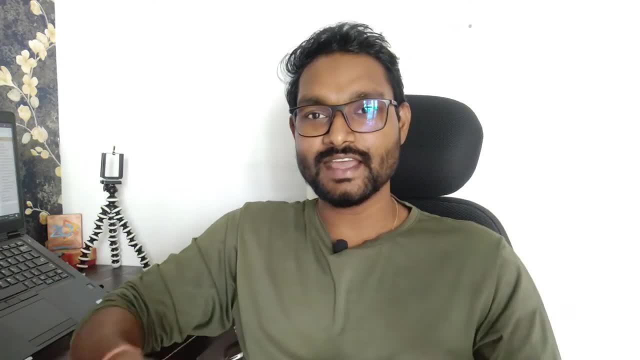 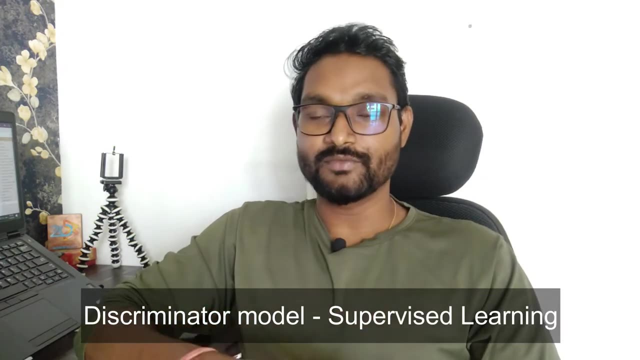 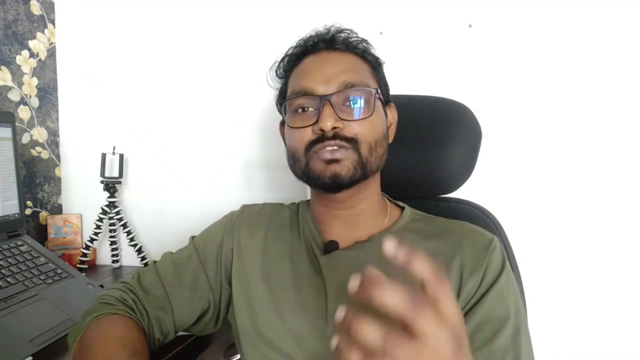 okay. so one more thing to notice over that: that inside of this GANs, the generative model is unsupervised learning model and the discriminator model is the supervised learning model because for discriminator model we used to pass whatever the output generated by the generator model and the actual sample images which we have, and this actual original sample image is labeled. 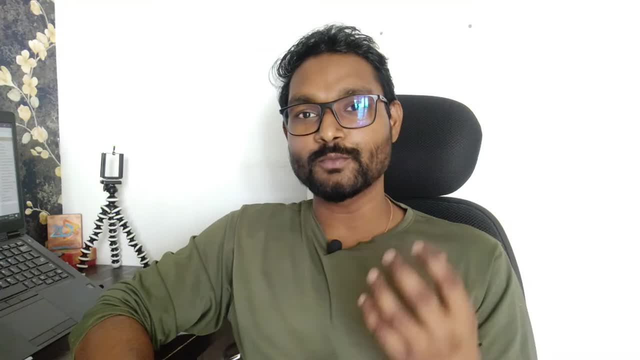 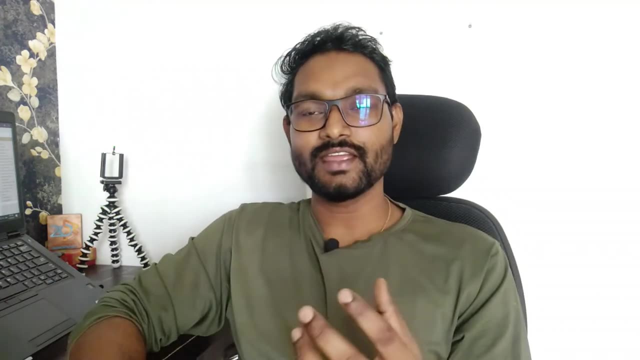 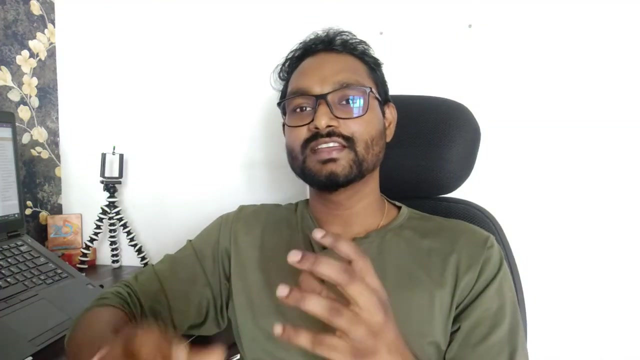 with original or the real, and whatever the output we generate from this generator model, we call that output as fake and label it with a fake and pass it to our discriminator model. and discriminator model's responsibility is to identify that whether past image is a real or fake means it is coming. 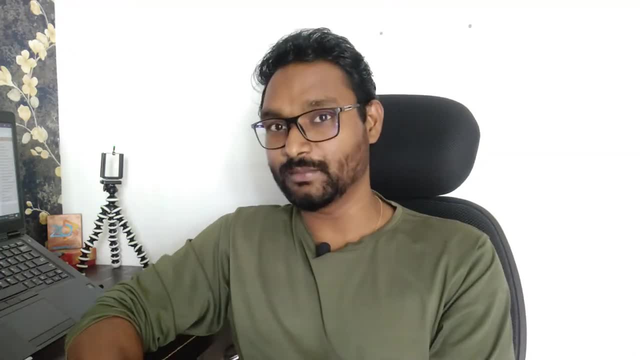 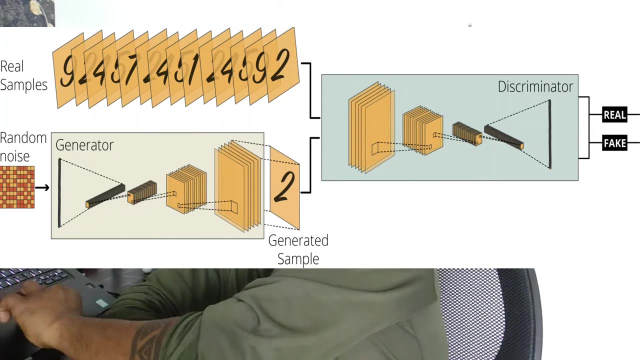 from our original data set or it was generated by the generator model. okay, so here you can see on the screen i have shown the generator and the discriminator model. okay, so you can see inside of this image. so at the left top you can see the real samples. okay, so here i am making a use of 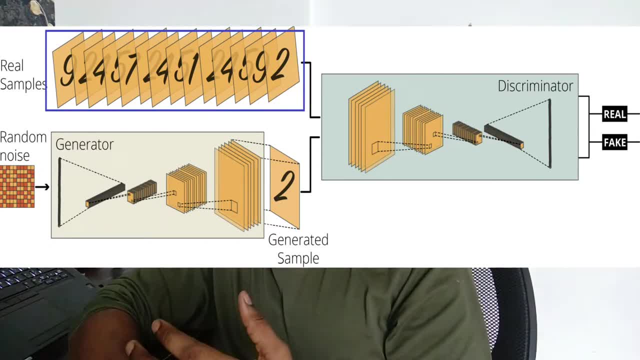 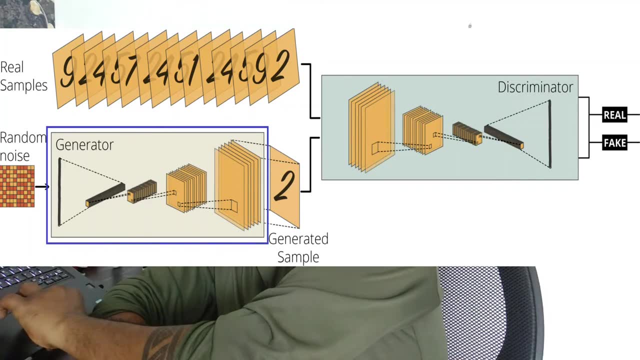 mnist data set and i am passing the all the images, handwritten images, from mnist data set to my model. just below to that you can see the generator model. so this block is showing like a generator model and it takes the random noise means any random input it takes and based on that, 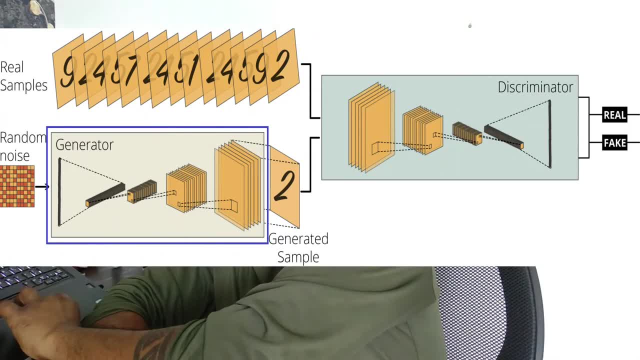 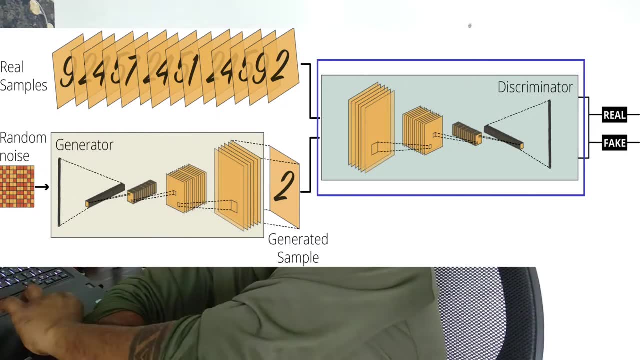 it generates some output. okay, and this generated output is nothing but the input for our discriminator model. so you can see, on the second part of this image we have a discriminator model. so whatever generated sample and whatever the real samples, we are passing it to our discriminator model. whatever is the 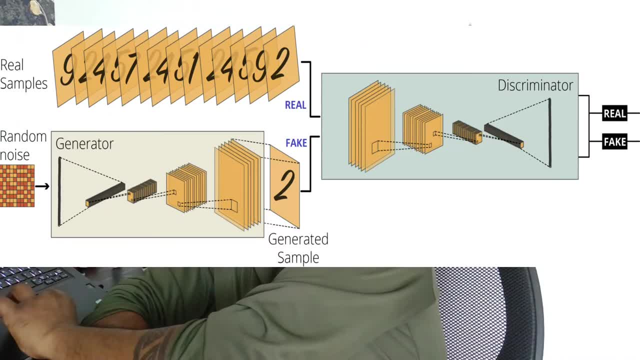 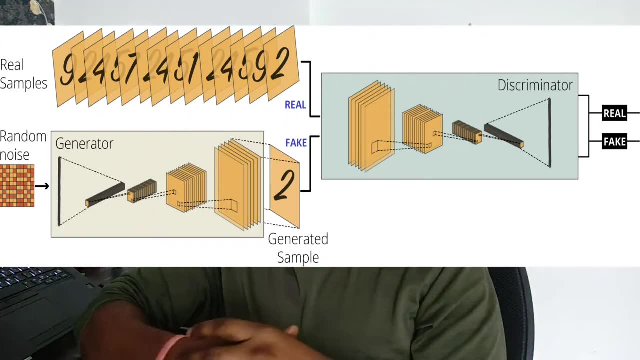 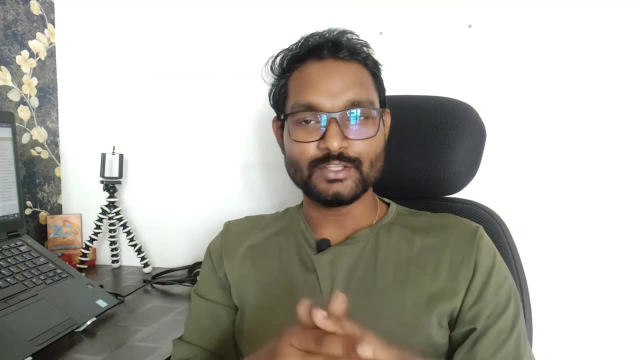 generated sample, we label it as a fake. and whatever the real sample, we label it as a real and pass it to discriminator model. and discriminator model learns from that and does the prediction whether the provided image is real or fake. okay, now you must understood about that GANs: having the two models inside of it. one. 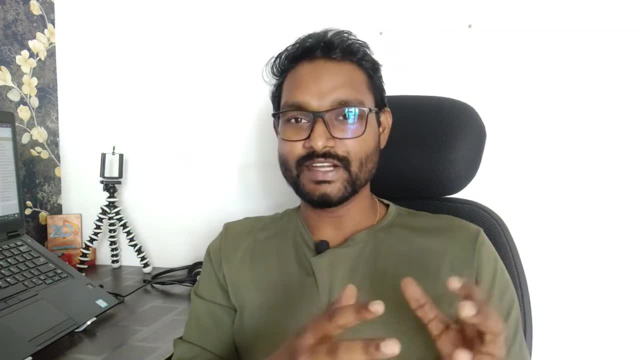 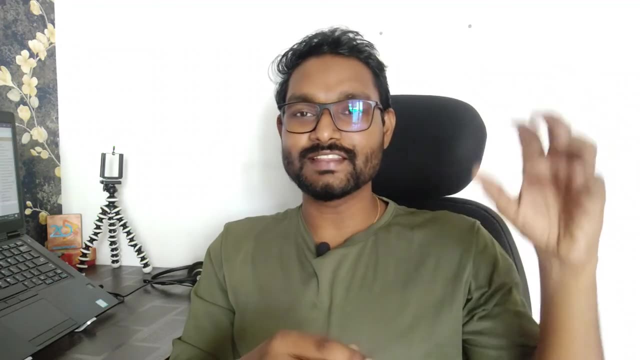 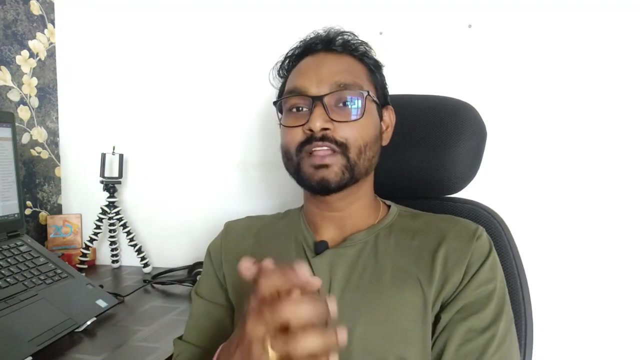 is a generator model and another one is a discriminator model. generator model takes a random input and generates one artificial output, and the discriminator model is responsible for taking the input of real and fake, and it does the classification: whether this image is real or fake. okay, now let's. 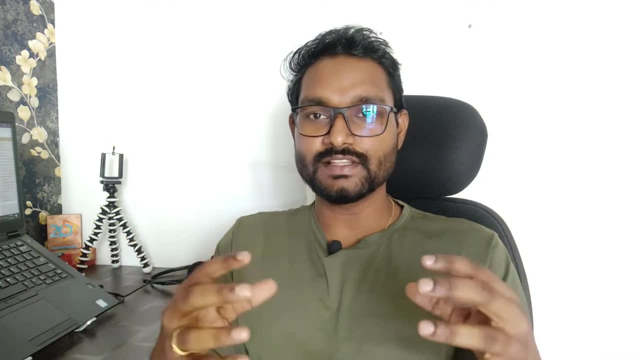 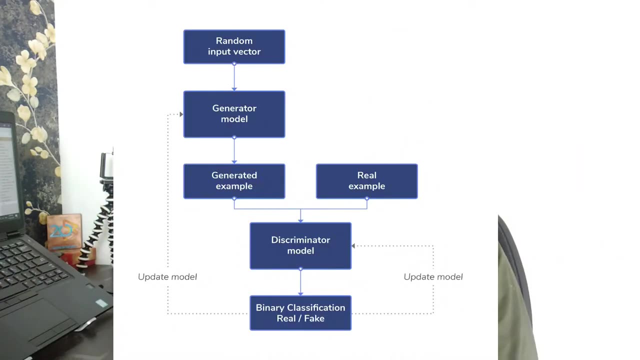 talk about how exactly this GAN works and how these two models inside of the GAN- generator and discriminator- work together and forms one generated adversarial model. so here you can see that I have shown another image and inside of that I have shown the simple flow. okay, 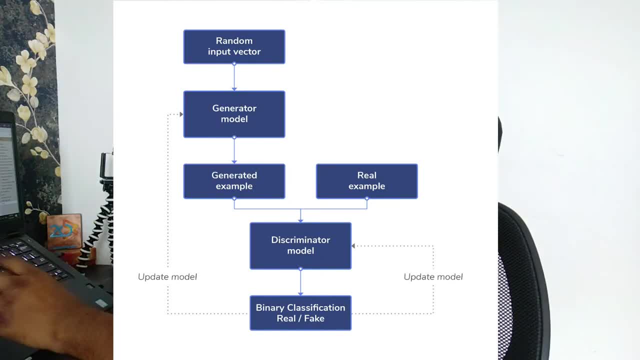 so this random input vector is the random input or the random noise we passed to our generator model and from that we generate one sample from this, while and this generated sample example and real example is passed to the discriminator model and discriminator model tries to identify whether pass. 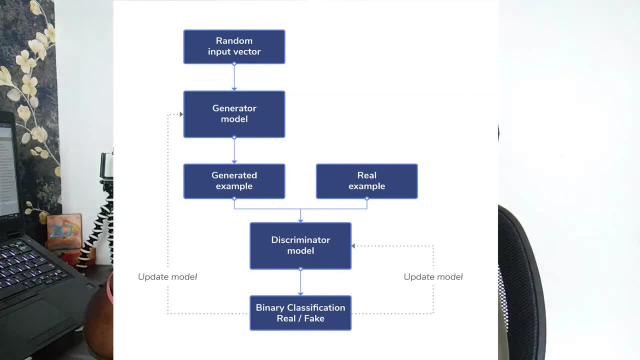 is artificial image which was generated by the generator model, or it is a real image which is coming from the data set. so it does the prediction and, whatever the real result comes in, based on that, it sends back a feedback to the generator model and the discriminator model. okay, so let's consider that we 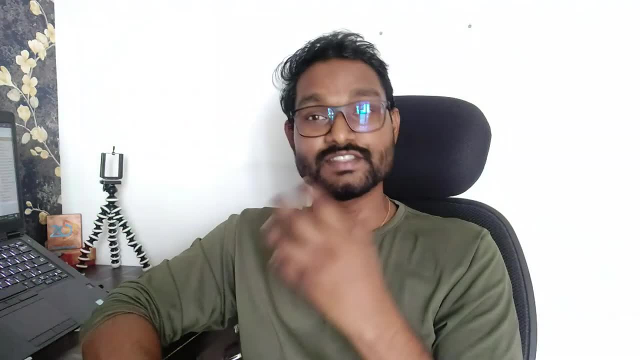 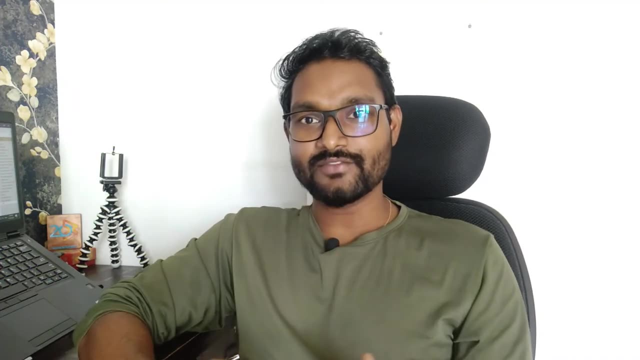 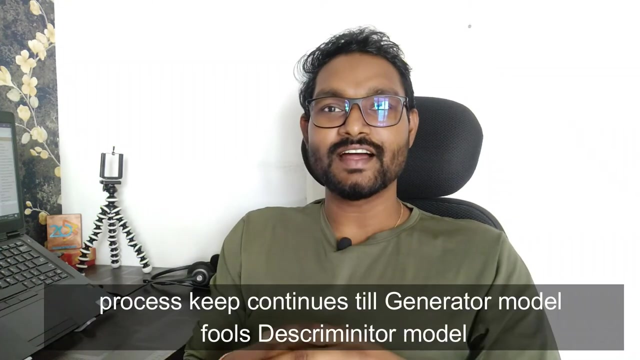 have generated an image from a generator model and pass it to our discriminator model, and discriminator model identified this fake image as a real, so in that case it will send back a feedback to both discriminator model as well as it will send to the generator model. this process keep continues until the. 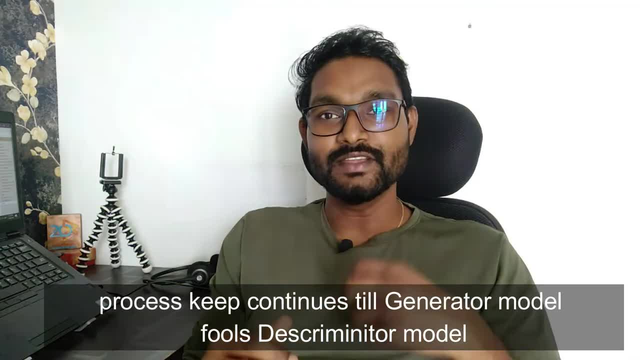 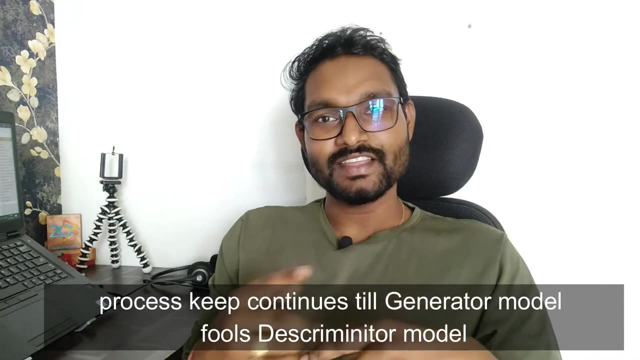 generated or the fake image is getting predicted as the real image by the discriminator. discriminator model when starts predicting the original image fifty percent as a fake and generated fake image as a fifty percent as original, till that case this model keeps running and keeps training and keep competitive. 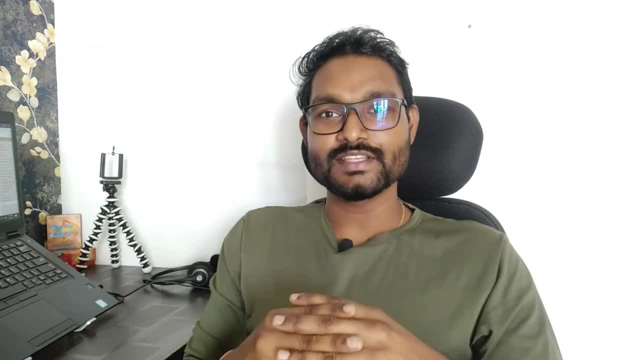 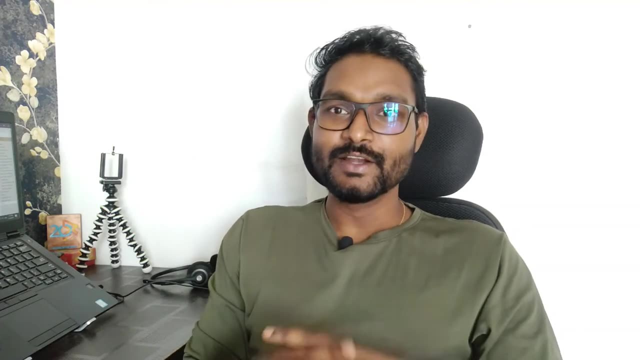 well about their geben art. so, as we are seeing, until the end of this model, we with each other. Once we got the 50% confidence for the real and fake, both images, at that time this model is good or considered as an ideal to generate a new image. Okay, so it means that 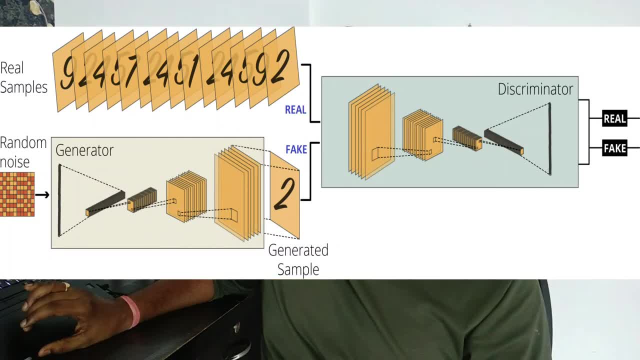 in our context. let's try to understand with the MNIST example. So let me go back to the example and here you can see that we are passing the real samples and the generator samples to the our discriminator model, and we are passing this- both images- along with a label like real image. 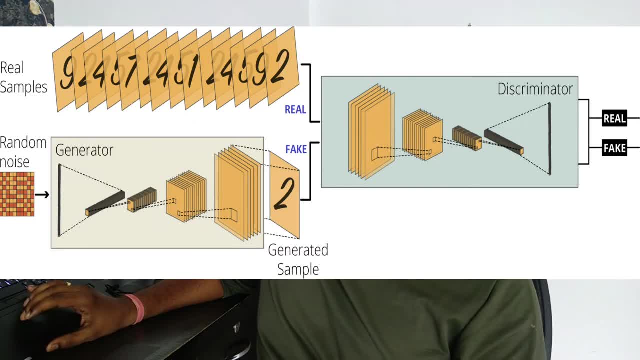 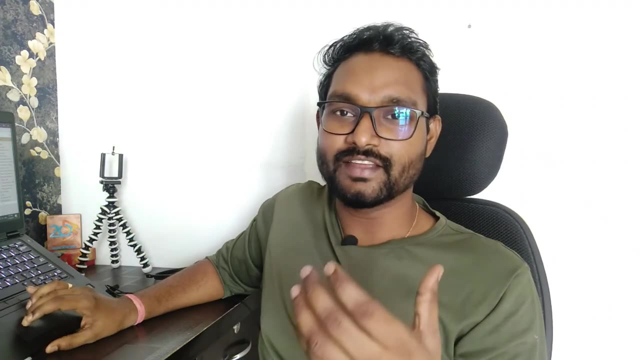 and the sample image. When discriminator model predicts, like a generated sample, as a real 50% time, it means that our generated image is successful in fooling the discriminator model. Okay, it means whatever image of handwritten character generator by the generator model that is that good that our discriminator model is not able to identify. 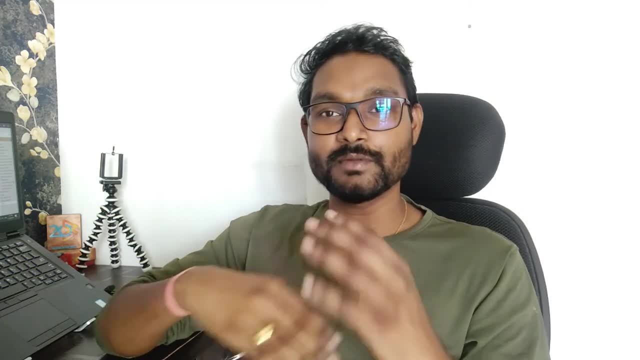 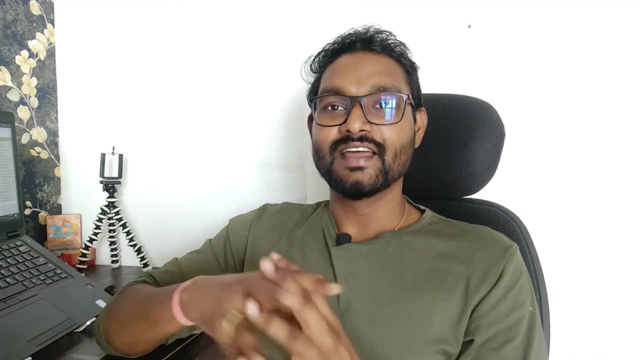 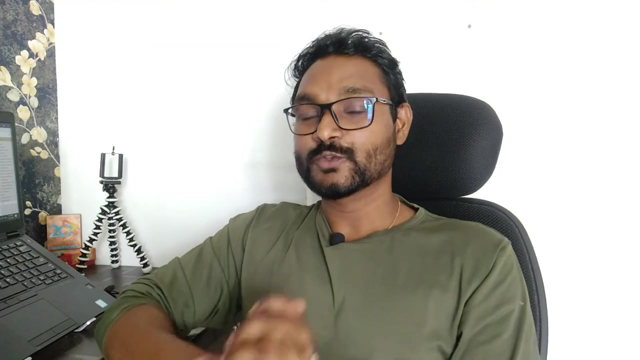 Whether it is a fake or original. it gets confused and 50% of time it is predicted the generated image- artificially generated image- as the original image. This is the ideal training of GAN, where we have proper competition between the generator model and the discriminator model. So this way: 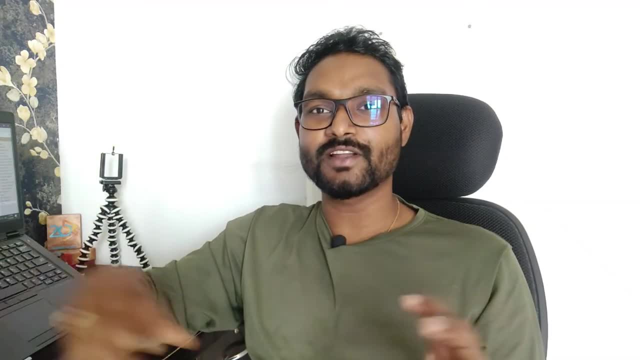 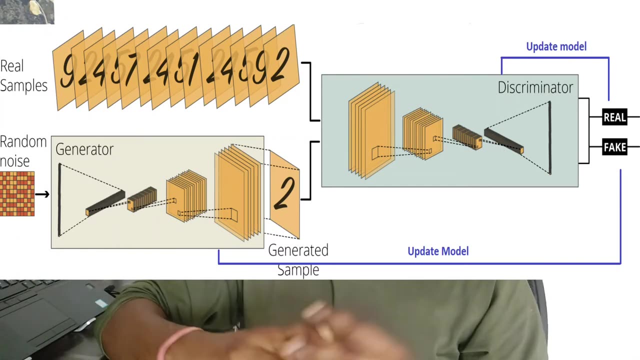 GANs are working with the help of a generator and discriminator model. Generator model generates a random output and again it goes to discriminator model and, based on the discriminator model's feedback, generator model generates a random output. So this way, GANs are working with the. 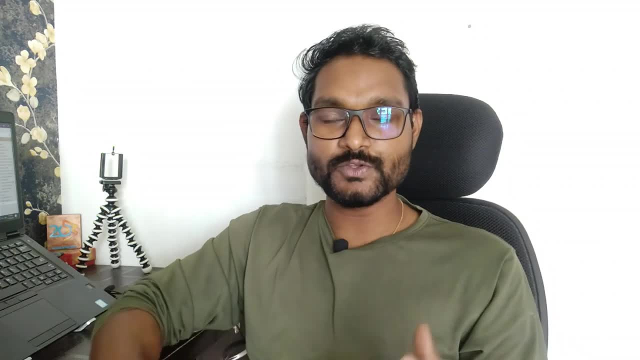 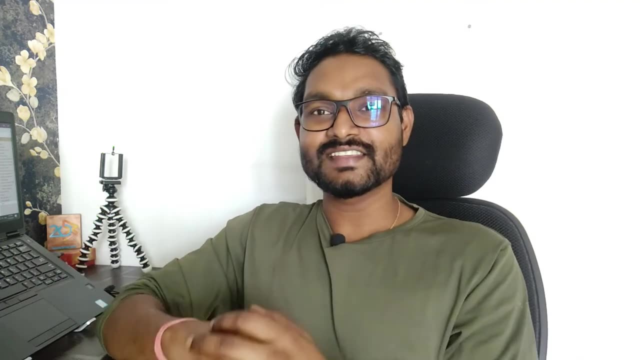 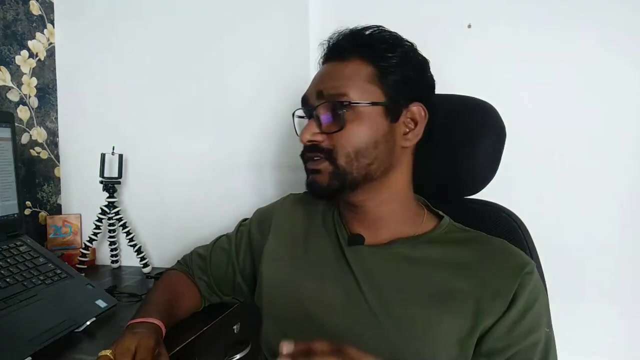 generator model and once the generator model starts producing the good image where our discriminator model starts identifying the fake image as a real, In that case our GAN is working good and it is able to generate the good handwritten digit images like a human beings. Okay, so this is. 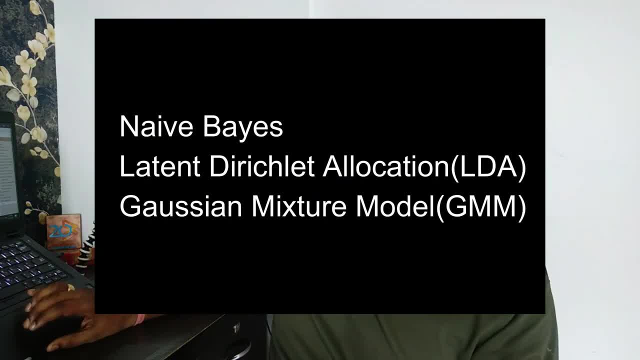 all about the working mechanism of the GANs, and now let's talk about. there are different examples of a GAN. One is a new bias, one after that the latent declut allocation and the Gaussian mixture model. Okay, so these are three examples of a GAN and one is a new bias, one after that the latent. 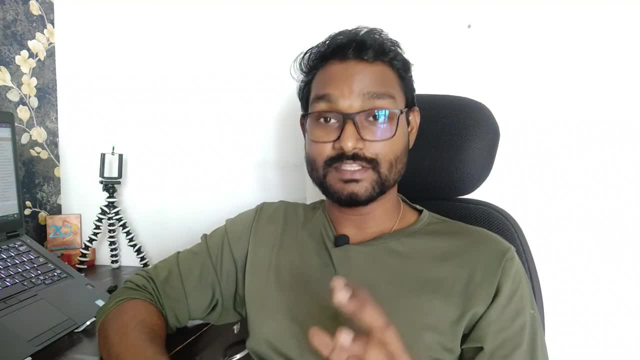 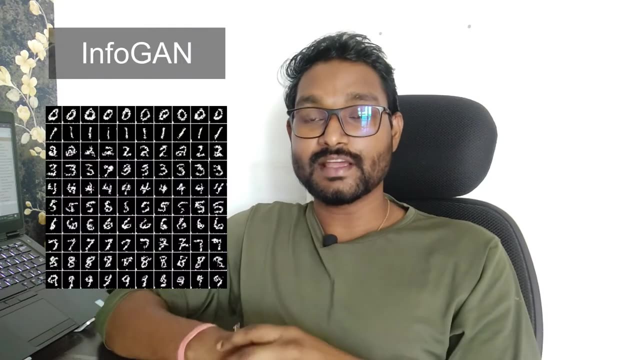 the examples of the GAN. So there are also different types of GAN based on its working mechanism, like SR GAN, Cycle GAN, Info GAN. So whatever the MNIST character example we are going to see in our next episode, that is falls under the Info GAN, that is, the Information Generative. 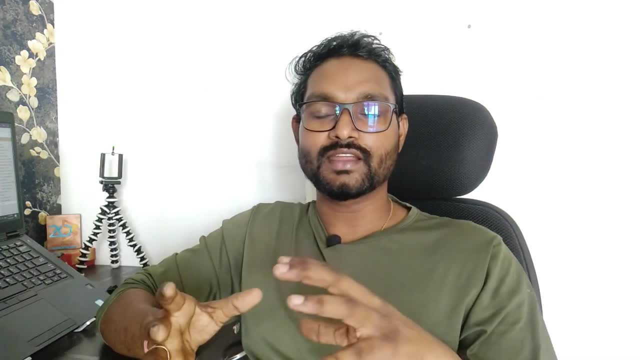 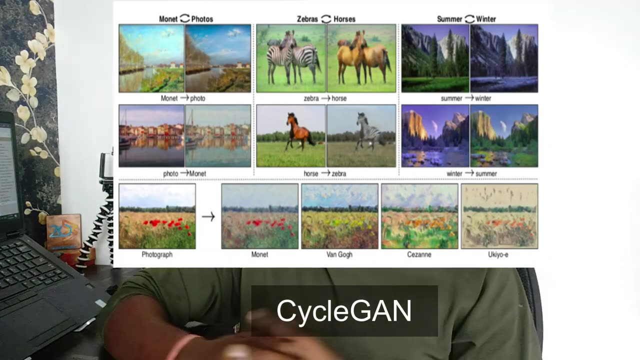 Adversarial Network. What are the images? I have shown that we can generate image of zebra from a horse and again we can generate a horse image from a zebra. So that is a Cycle GAN and there is a SR GAN where we can do the combination of different images and produce a new one. 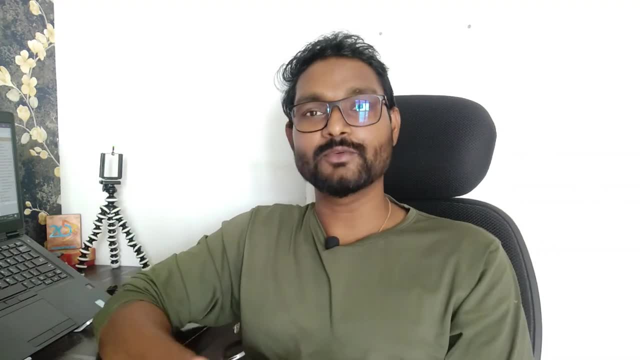 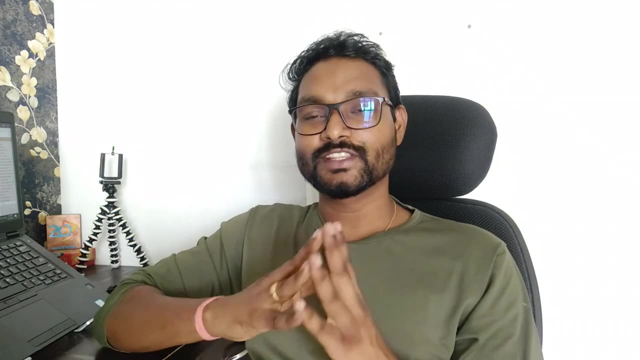 Okay, so these are three major types of the GAN. There are other also, So I am going to provide the link in the description box. You can go through that and you can learn more about the different types of a GAN. Okay, so that's it for today's episode, where we have talked about 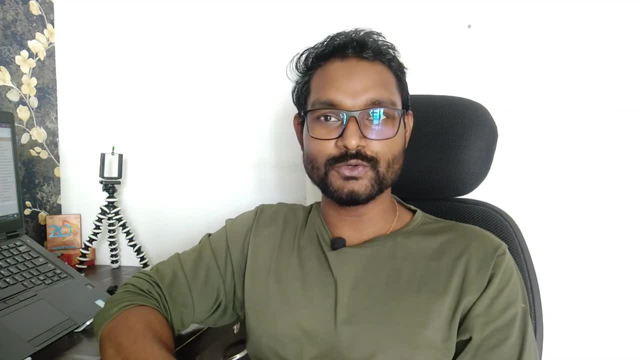 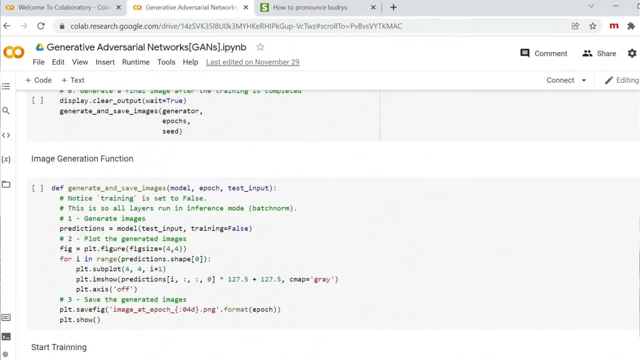 intuition, part of the GANs, and in our next episode I am going to show you the actual implementation of GAN, where we develop our generator model, we will develop a discriminator model and we will apply on the MNIST data set And we will try to generate a new handwritten, artificial handwritten digits which are similar. 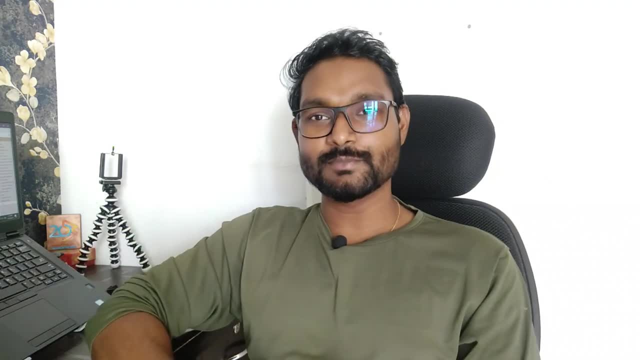 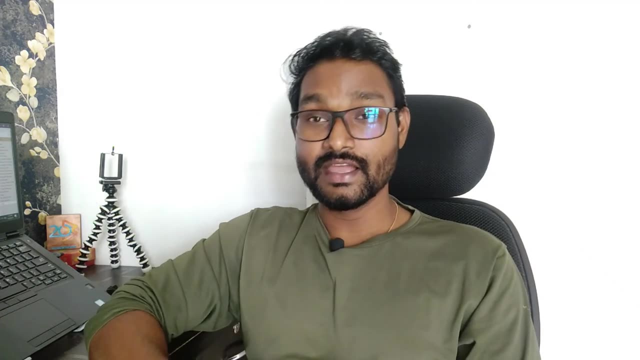 like the human rights on the paper. Okay, so that's it for today's episode. Hope you like this information. If yes, then please hit on the like button. Subscribe to this channel to learn more about data science and machine learning If you have any questions or doubt.